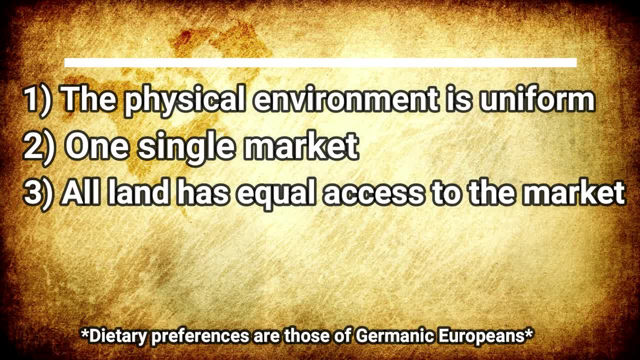 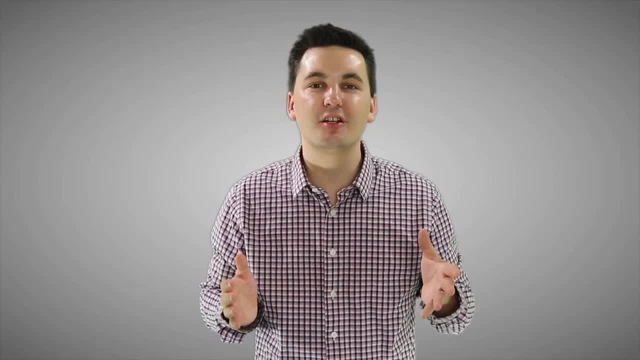 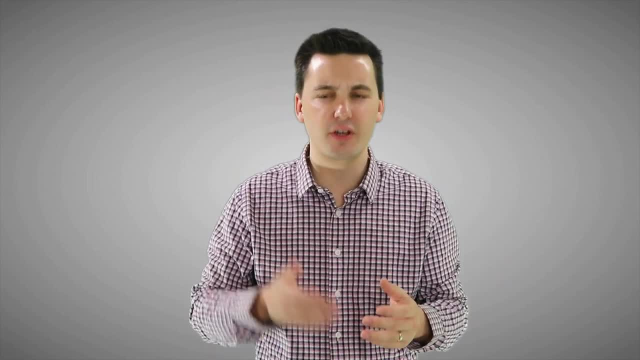 and that all land has no land. The model also assumes that farmers want to maximize their profits and that all land has similar site characteristics. Now I can already hear some of you in the comments section saying: Mr Sin, this doesn't make sense. The physical geography is not all the same. We have different climates, different amounts of arable land. 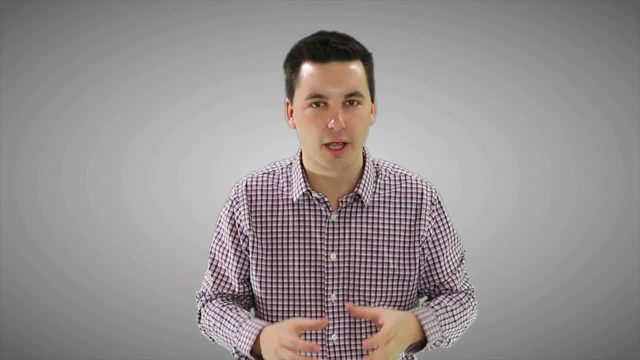 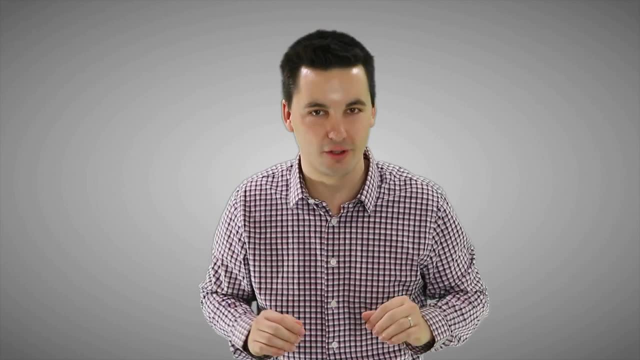 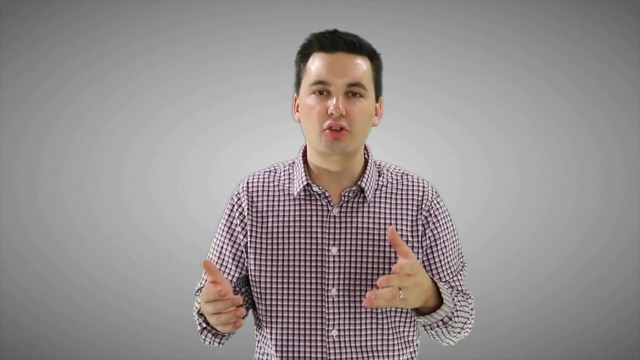 We trade in a global community. We don't stay in an isolated area. We have new technology that changes how we produce food, And we'll get to all of these concerns, I assure you later in this video. However, remember Models are simplified versions of reality. They're not a perfect match. Vom Tunin used these assumptions so this model could be applied to different geographic areas. 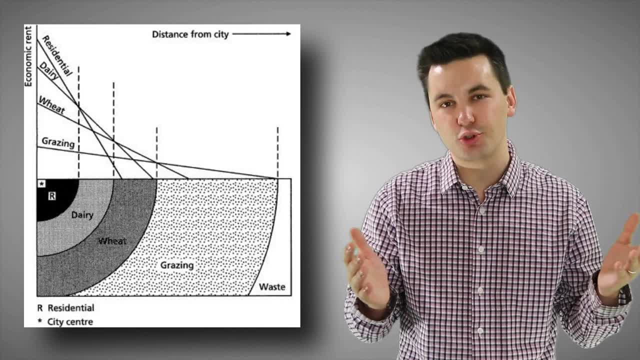 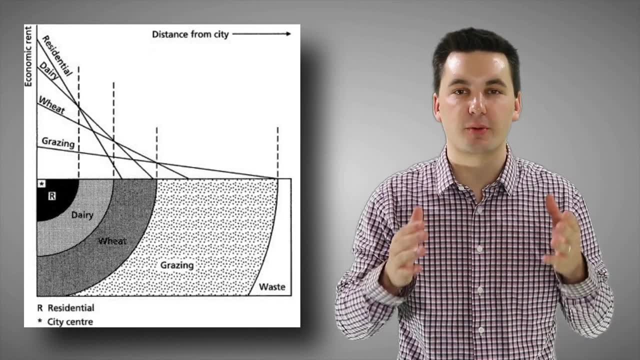 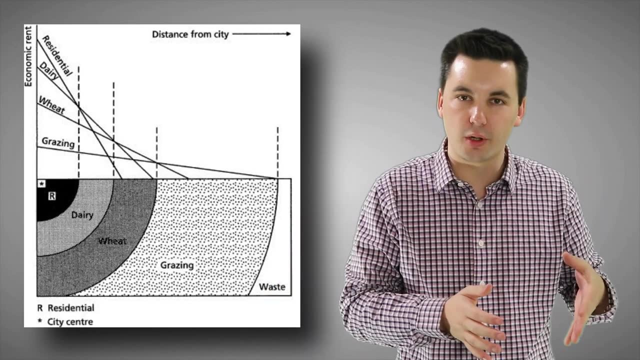 Now it's almost time for us to go over his model. But before we get into that, I need to make sure you remember the bid-rent theory. We talked about this in the Unit 5, Topic 6 video. Remember the bid-rent theory looks at the value of land. As we move farther away from an urban area, the price of land goes down. As we move closer to an urban area, the price of land goes up. Remember the bid-rent theory looks at the value of land: As we move farther away from an urban area, the price of land goes down. As we move closer to an urban area, the price of land goes up. Remember the bid-rent theory looks at the value of land: As we move closer to an urban area, the price of land goes down. As we move closer to an urban area, the price of land goes up. 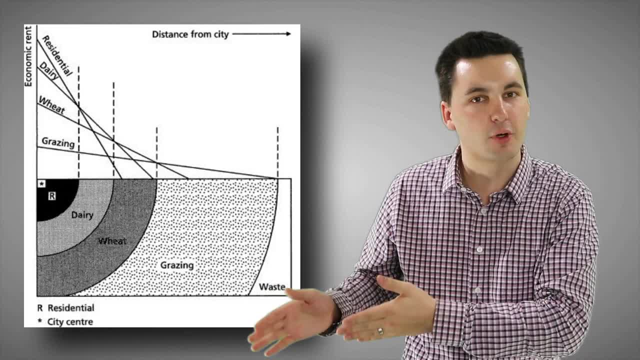 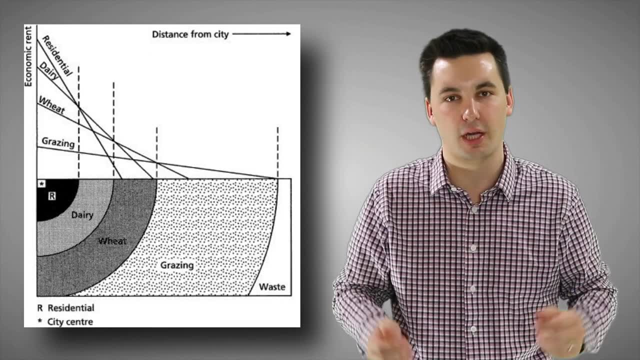 Remember, we're more likely to see extensive agriculture be practiced further away from a market area or an urban area, And we're more likely to see intensive agriculture be practiced near an urban area, And all of that has to do with the price of land. That's going to be important to understand when trying to understand Vom Tunin's model. 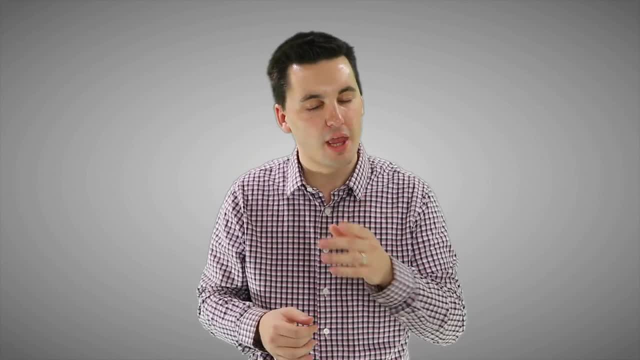 And if you don't remember extensive agriculture, intensive agriculture or that bid-rent theory, go check out my 5.6 video and then come back and finish this one. That way the Vom Tunin model will make sense to you. 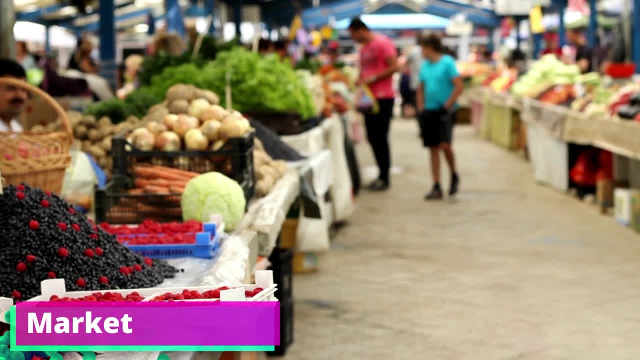 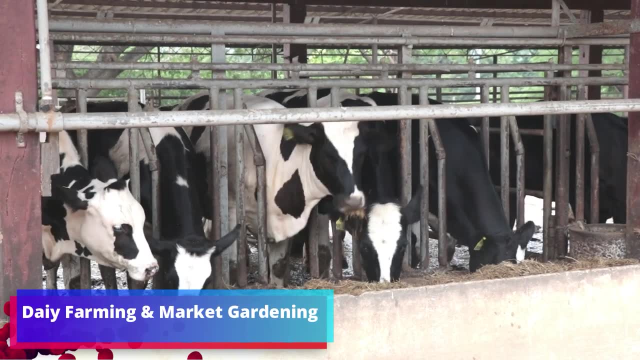 At the center of Vom Tunin's model was the market. At the center of Vom Tunin's model was the market. Here was where the agricultural crops and products would be sold to consumers. Now, as we move outward from the market and into the first ring outside the market, we would find dairy farming and horticulture. 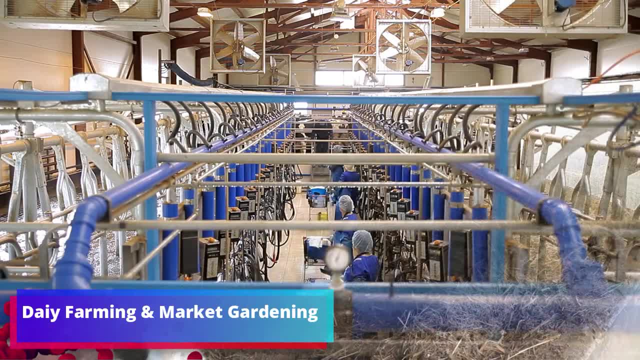 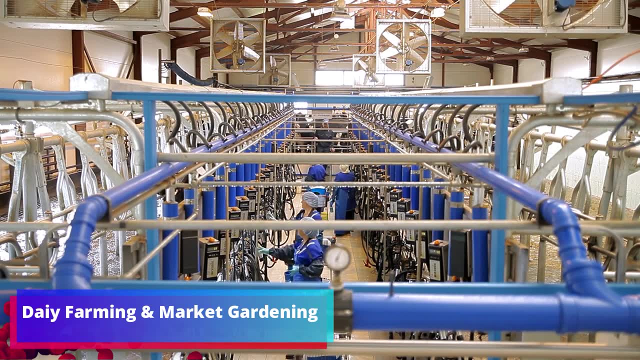 Which is located next to the market, because the goods are perishable. Remember, Vom Tunin created this model before the Industrial Revolution, which means we didn't have refrigeration. These products have a higher transportation cost, partially because of the speed needed to get them to the market. 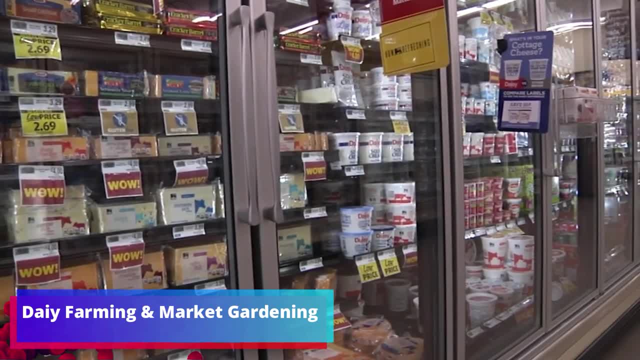 If they don't reach the market, they won't be sold. If they don't reach the market, they won't be sold. If they don't reach the market fast enough, they'll spoil and go bad At the same time. these products require less land to produce. 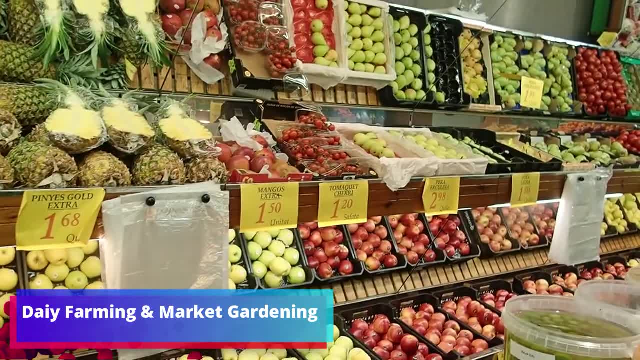 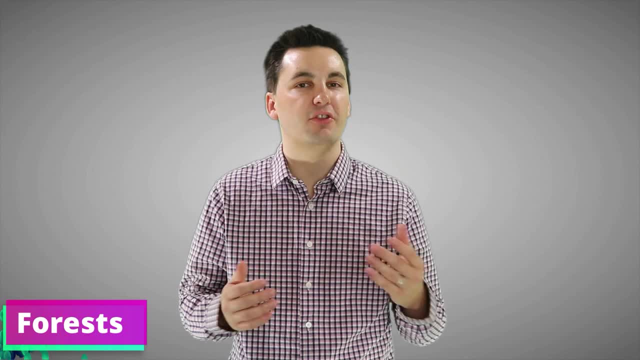 So by having dairy and horticulture next to the city or the market, we can maximize our profits and minimize our costs. The next ring is the forest, which today doesn't make as much sense, But at the time lumber was used to build homes, heat homes, cook food. it was essential for people. And lumber is very difficult to transport. It's bulky, it's heavy, and so transportation costs, if located too far away, would be too high. So the forest was located in that next ring to allow for it to be able to get quickly to the city and reduce those costs. 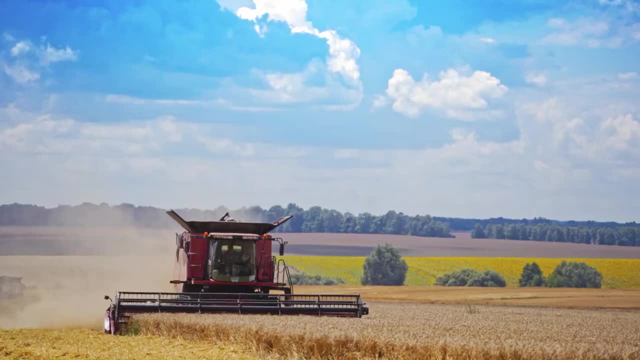 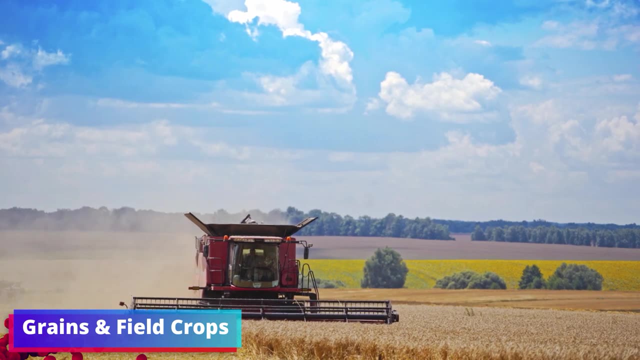 Again, remember: this model is all about maximizing our profits. Going into the third ring, we can see grains and field crops. These crops are lightweight, They don't perish and are easy to transport. This makes them cheaper to transport, so they don't need to be close to the market. 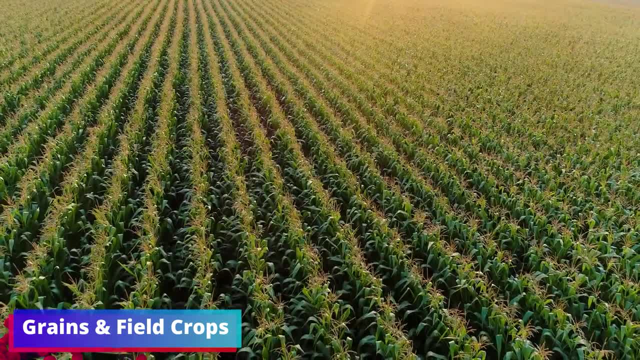 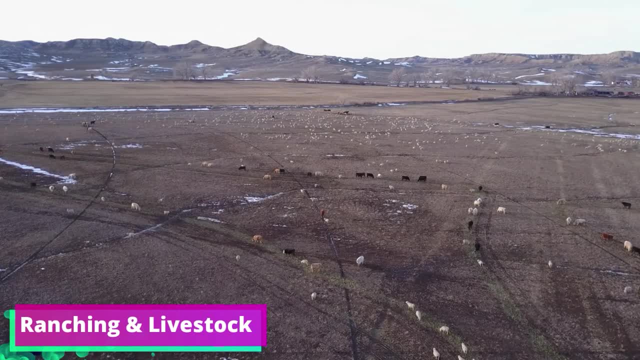 These crops also require more land, So by locating them further from the market we can reduce our costs, since land is cheaper. You can see the bid-rent theory is epic. The last ring is livestock or ranching and livestock. It's located here because of the amount of land needed in order for the livestock to graze. 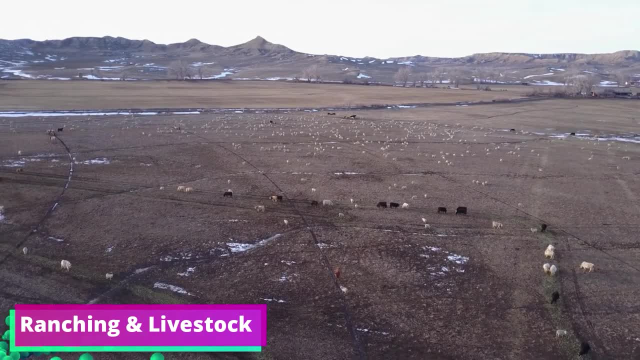 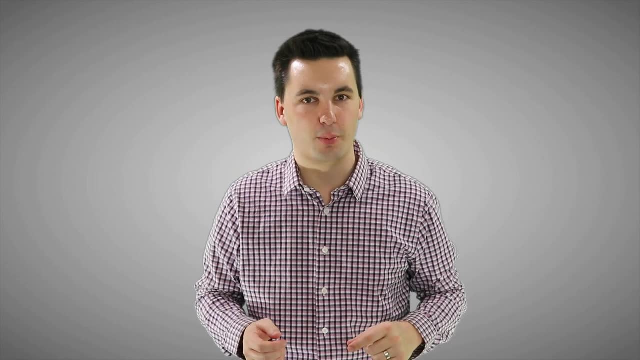 It would be difficult to acquire so much land near the market due to the cost of the land. Now, the one issue that some of you may have noticed is that meat is perishable. It's also not the lightest thing to transport, So the further away it is from that market, the more expensive it is to transport. 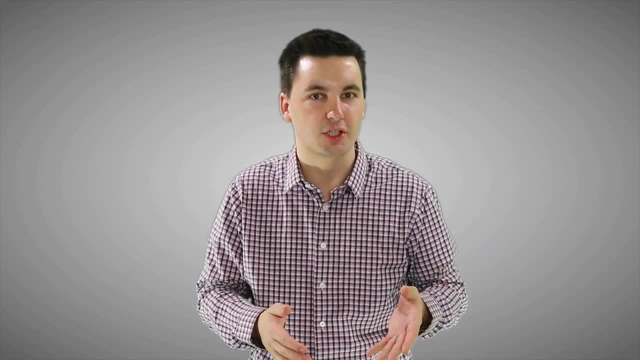 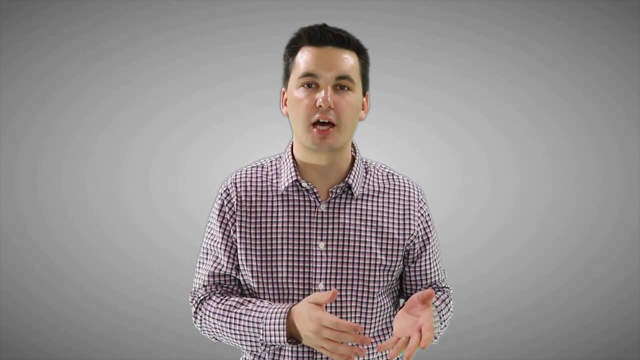 And so some of you might be asking: well, why isn't this within the dairy production? And honestly, it's a great question. The reason why livestock is so far out from the market is because the animals can walk themselves to the slaughterhouses that can be closer to the market. 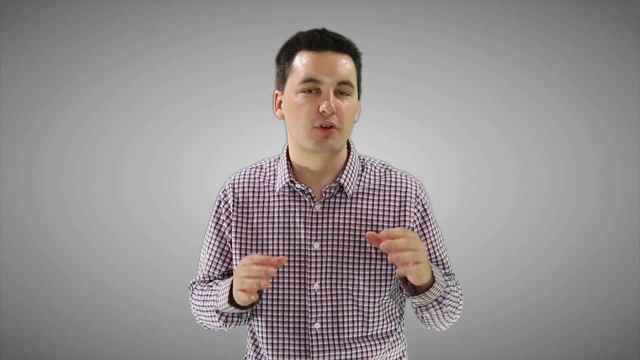 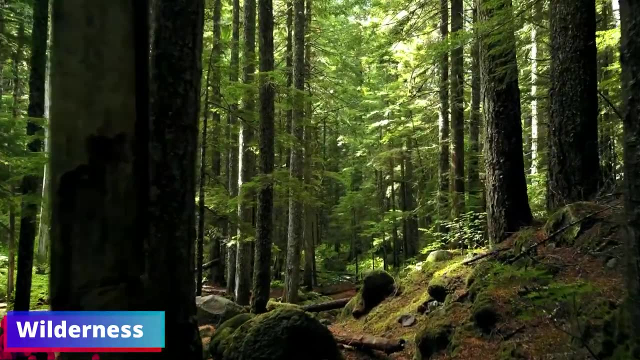 This allows farmers to get the cheaper land rates and also reduces their transportation costs. And if we move past the last ring, we'll find ourselves in the wilderness, And that's because we're too far away from the market for any commercial agriculture to be profitable. 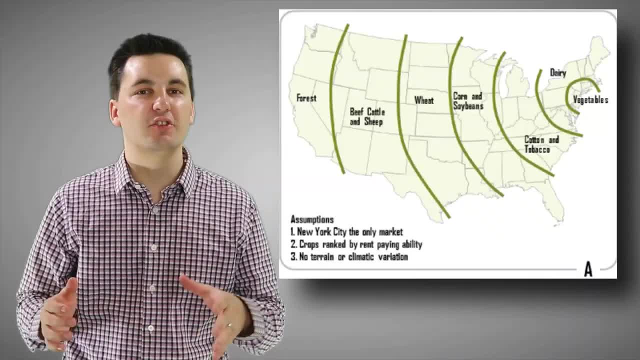 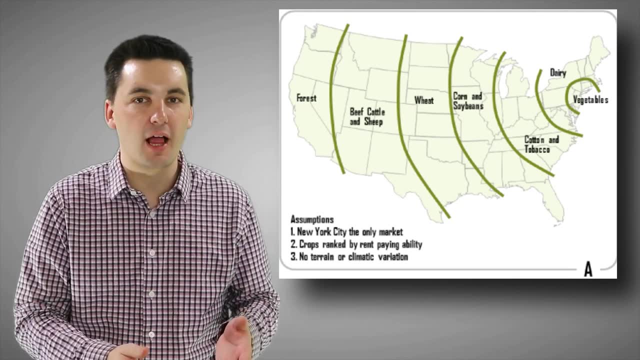 So we wouldn't see any located this far away from that urban center. Today we can see that many parts of von Thunen's model still apply to society today. However, some parts have started to change due to advancements in technology and shifts in society.